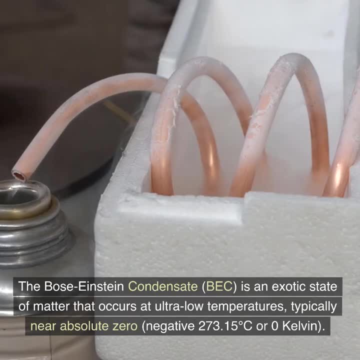 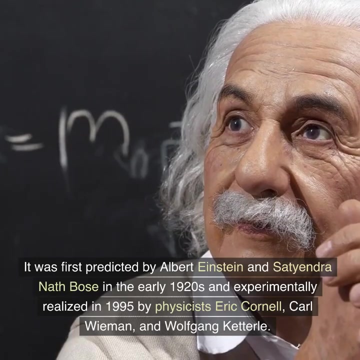 The Bose-Einstein condensate BEC is an exotic state of matter that occurs at ultra-low temperatures, typically near absolute zero negative 273.15 degrees Celsius or zero Kelvin. It was first predicted by Albert Einstein and Satyendra Nath Bose in the early 1920s and 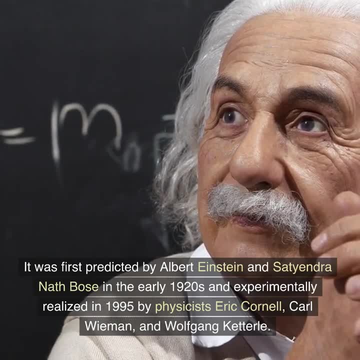 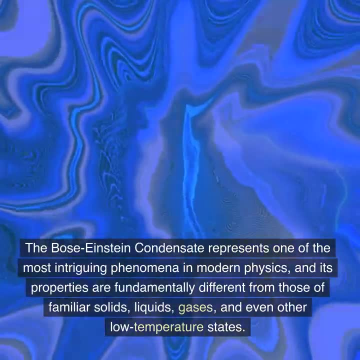 experimentally realized in 1995 by physicists Eric Cornell, Carl Wieman and Wolfgang Ketterle. The Bose-Einstein condensate represents one of the most intriguing phenomena in modern physics, and its properties are fundamentally different from those of familiar solids. 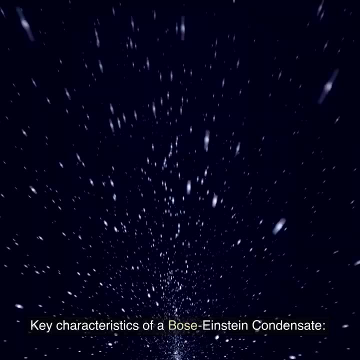 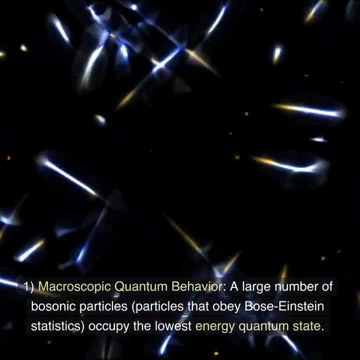 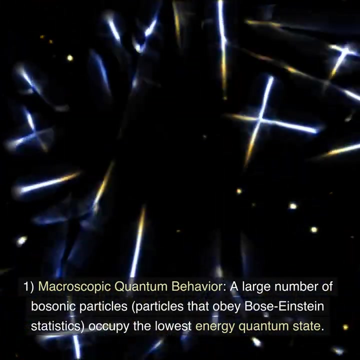 liquids, gases and even other low-temperature states. Key Characteristics of a Bose-Einstein Condensate: 1. Macroscopic Quantum Behavior: A large number of bosonic particles, particles that obey Bose-Einstein statistics, occupy the lowest energy quantum state. 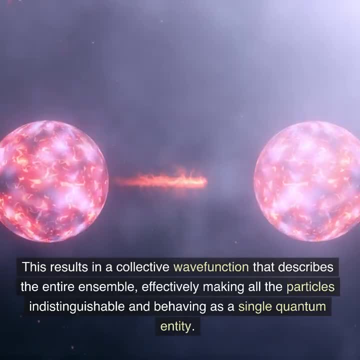 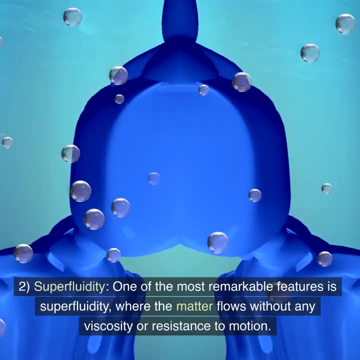 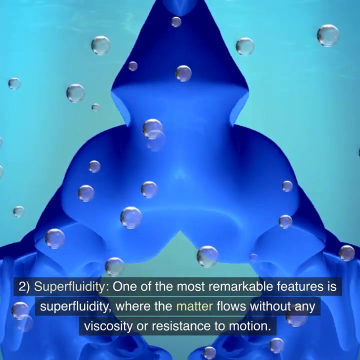 This results in a collective wavefunction that describes the entire ensemble, effectively making all the particles indistinguishable and behaving as a single quantum entity. 2. Superfluidity: One of the most remarkable features is superfluidity, where the matter flows without any viscosity or resistance to motion. 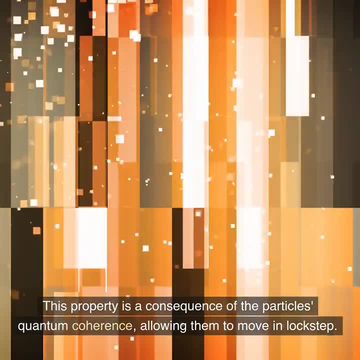 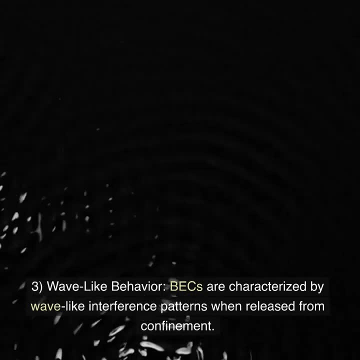 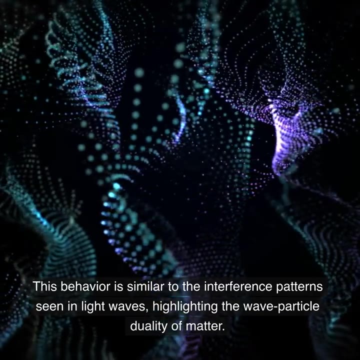 This property is a consequence of the particles' quantum coherence, allowing them to move in lockstep. 3. Wavelike Behavior. BECs are characterized by wave-like interference patterns when released from confinement. This behavior is similar to the interference patterns seen in light waves. 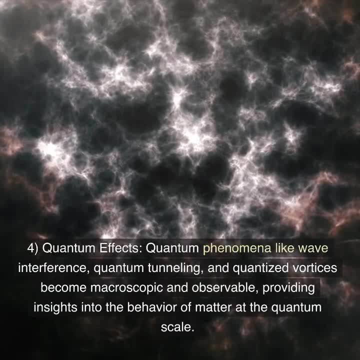 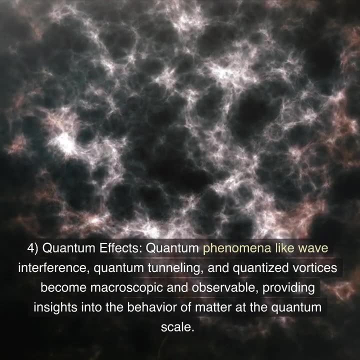 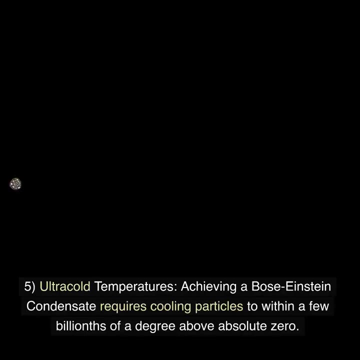 highlighting the wave-particle duality of matter. 4. Quantum Effects: Quantum phenomena like wave interference, quantum tunneling and quantized vortices become macroscopic and observable, providing insights into the behavior of matter at the quantum scale. 5. Ultra-Cold Temperatures. 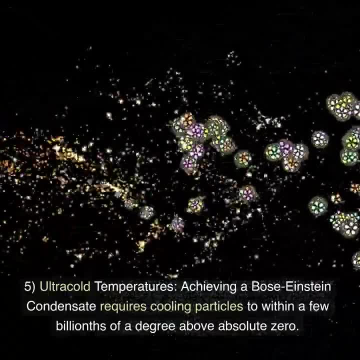 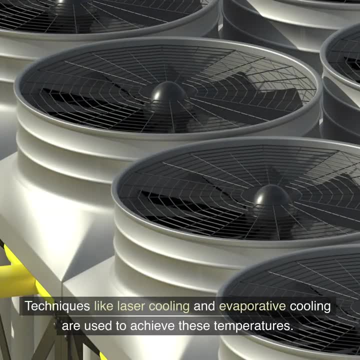 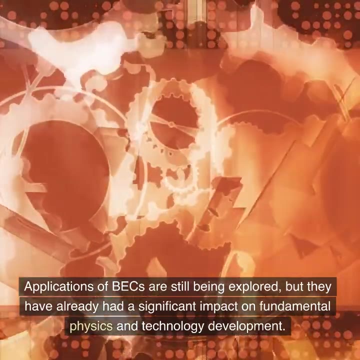 Achieving a Bose-Einstein condensate requires cooling particles to within a few billionths of a degree above absolute zero. Techniques like laser cooling and evaporative cooling are used to achieve these temperatures. Applications of BECs are still being explored, but they have already had a significant impact on fundamental physics and technology development.